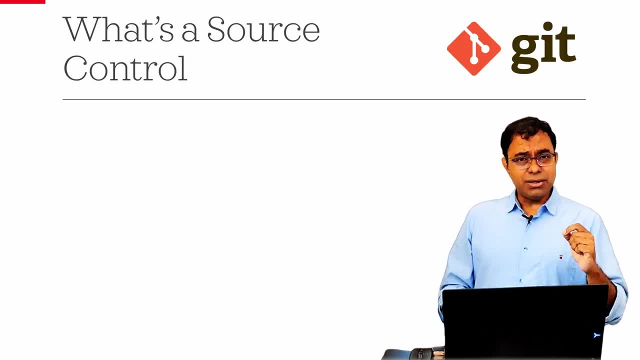 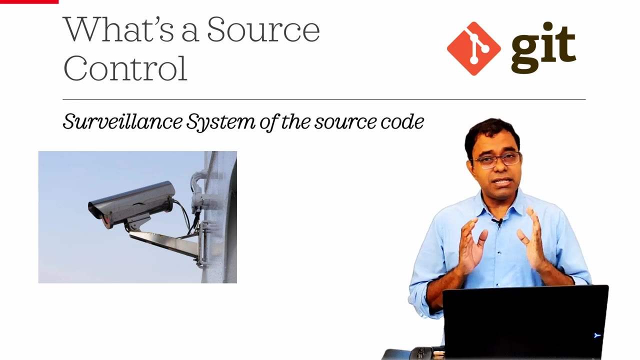 so, before going ahead and talking about Git, let's talk about source control. What is a source control? This picture should look familiar to you, right? You have a CCTV camera for surveillance. So source control is nothing but a surveillance system of your source code. right, A source? 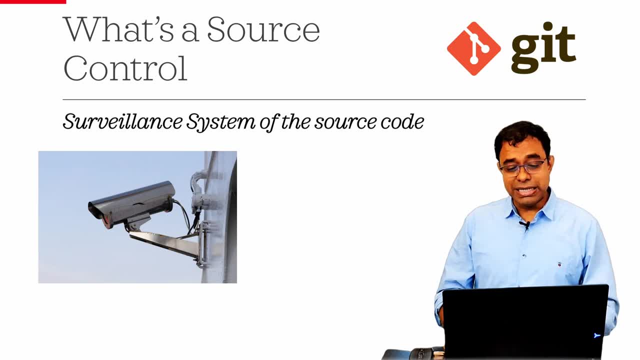 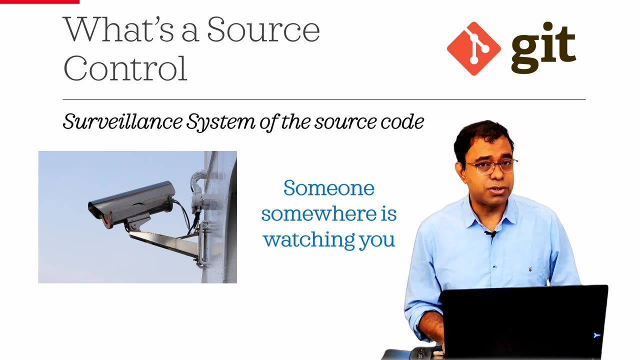 control is a surveillance system of your source code, which means someone somewhere is watching you, not you your source code using your source control. Okay, so it's very similar to a surveillance system for your source code. Now the source control tools are also called version. 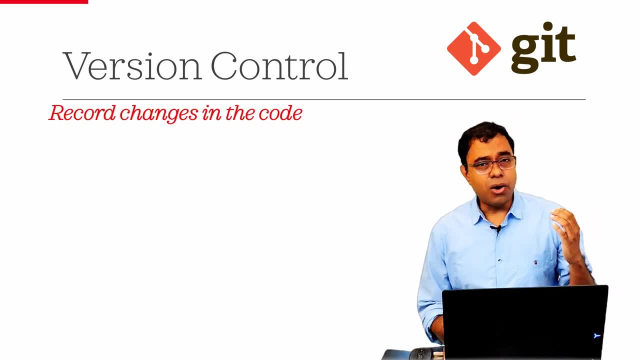 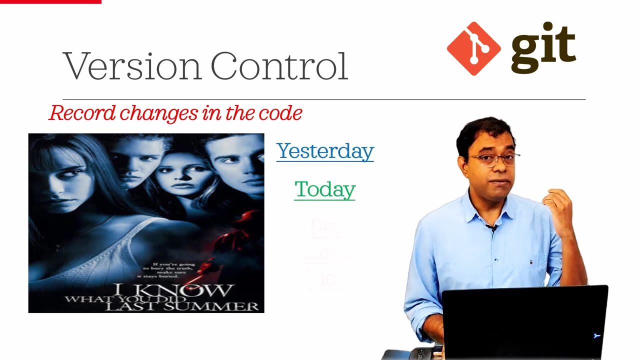 software. So version control is all about recording changes in your source code, which means I know about your source code, which means I know what you did last summer, or yesterday or today or even few seconds back. This is what version control gives you to your source code. Now the question. 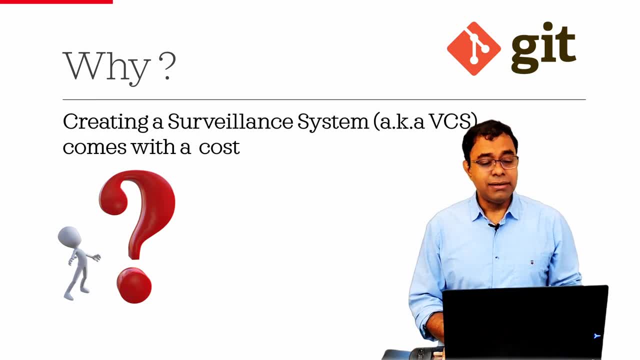 you must be asking why. Why do I need this? Because creating a surveillance system, aka version control system, comes with a cost right. Any tool cannot be created without investing anything right And implementing it. getting the system up and running, training all the people in it, takes time and cost. Why do we use it? The answer: 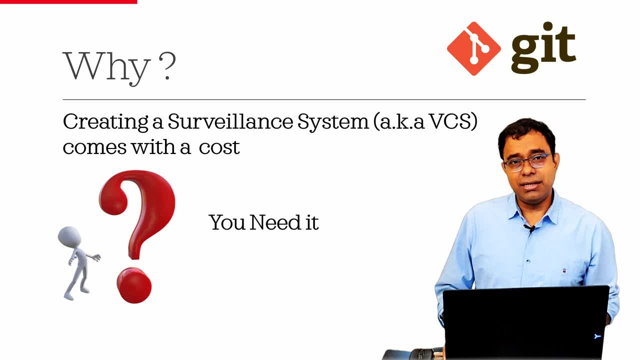 is: you need it. There is no other answer. Go ahead, try a source control software and then come back and say that you don't need a source control. If you have a genuine reason for saying that, believe me, you will end up in Guinness Book of World Records. Okay, because there are no. 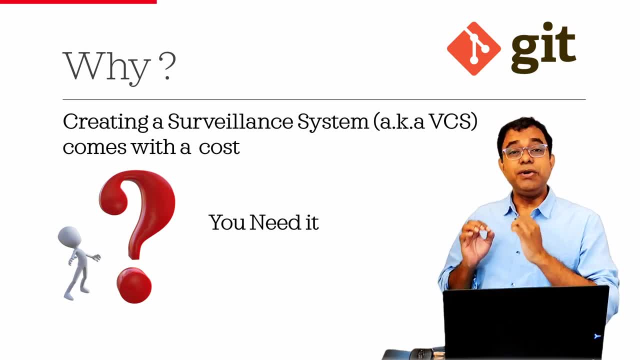 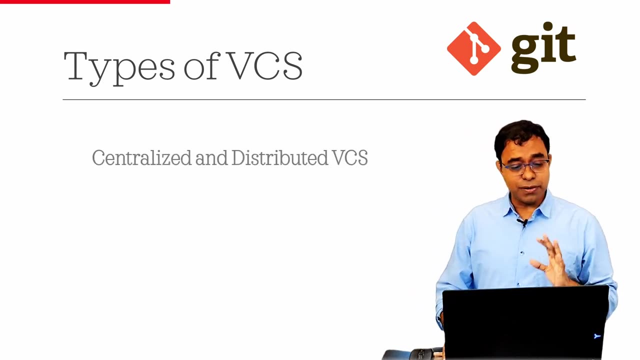 programmers, no software engineers, can say that we don't need source control. You need source control. Go ahead, use it and you will understand yourself why. Okay, so now let's talk about types of version control system. There are two types of version control systems. There are two types of. 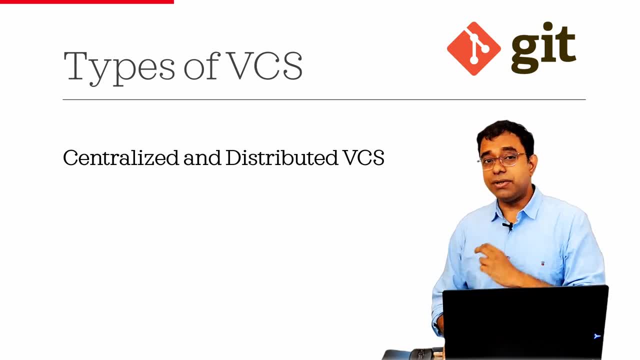 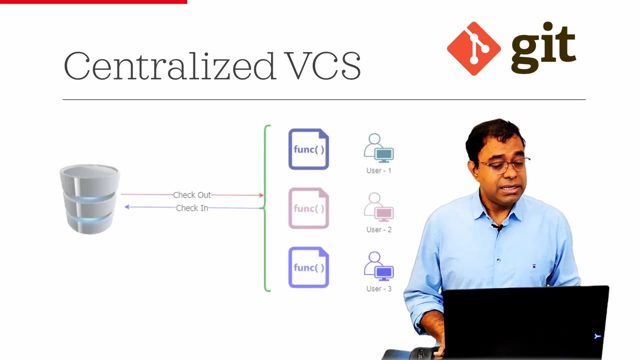 version control system called centralized as well as distributed version control system. SVN is a centralized version control system and Git is a distributed version control system. Now let's understand what is the meaning of this centralized and distributed version control system. Centralized version control system means your source code and all the information about I know. 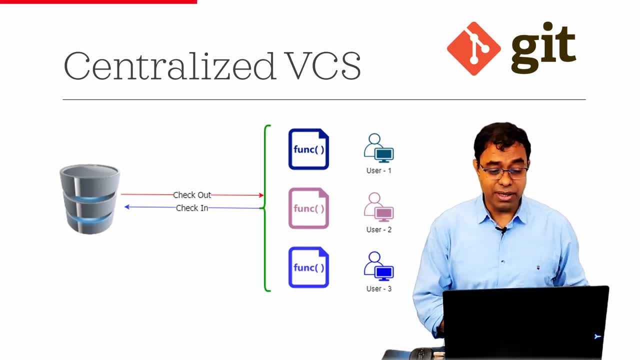 what you did last summer stored in a server. Okay, whenever one user wants to work on that, it checks out the file and after the working it checks in the file. there is nothing that is stored in the user's local system. That is called centralized version. 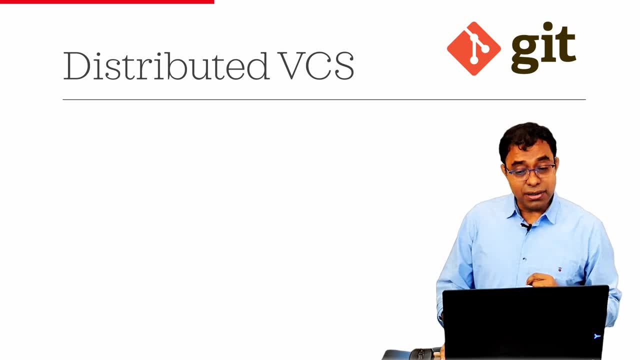 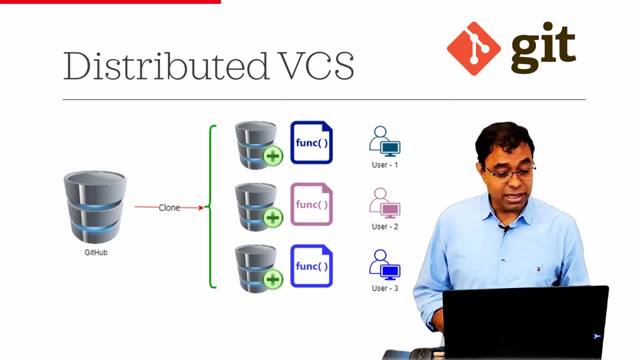 control system like SVN, Distributed VCS, which is Git, works in this way. Consider your centralized server: is GitHub. Okay, you clone the repo, which means that the exact replica of everything comes to your local system And you are working on your local system. So the history of I know what you did yesterday or today. 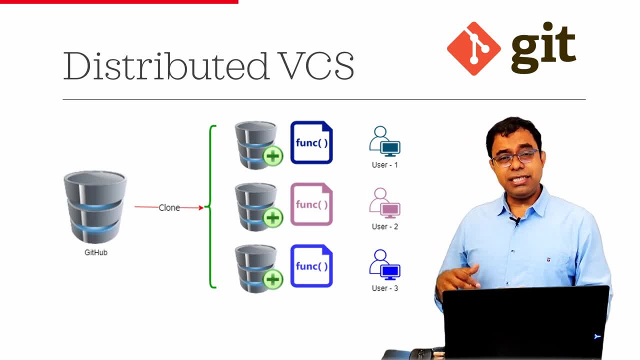 is actually stored in your local system. This means that you can consider a source control in your local system and you don't need to be connected to GitHub to you know. go ahead and start working on it, checking out and checking in your file, and changes, Of course, after doing it. 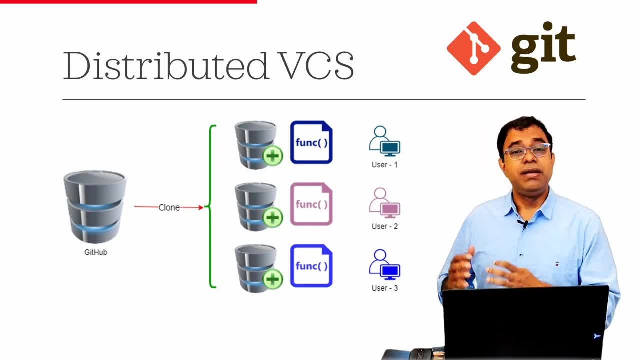 you can put it back to GitHub At some moment of time, but right now you can do it without connecting to GitHub because you have cloned the repository. There are some limitations of getting the history of complete history, but still we are not going to talk about that right now. This is what distributed version control. 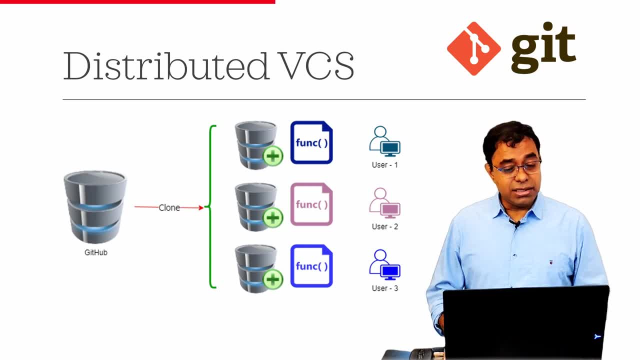 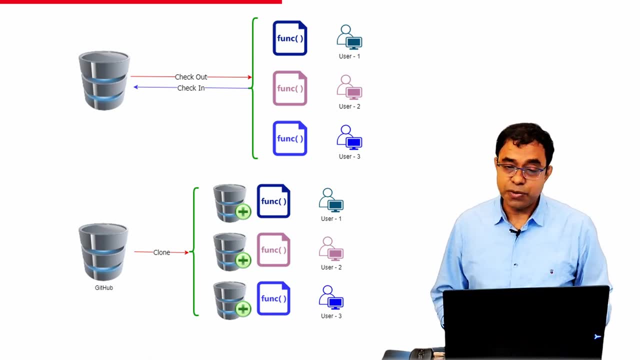 system means and this is what Git is. So let's see side by side. The top one is centralized version control system. The bottom one is distributed version control system. You understand the difference. in centralized version control system. Nothing comes in the user system and user. 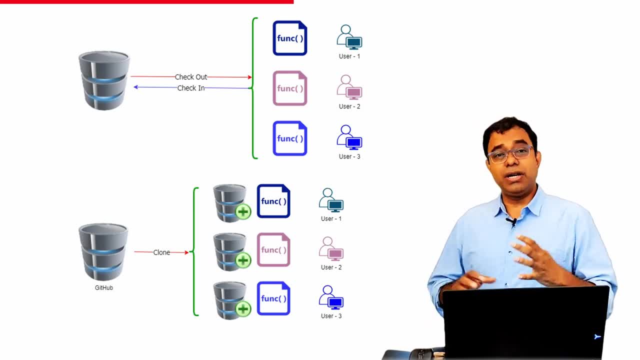 cannot work on the file. Work means that you cannot check in back your changes until unless you are connected to the centralized version control system, which is not required in Git. Now we understood that Git is a distributed version control system. Let's talk about one of. 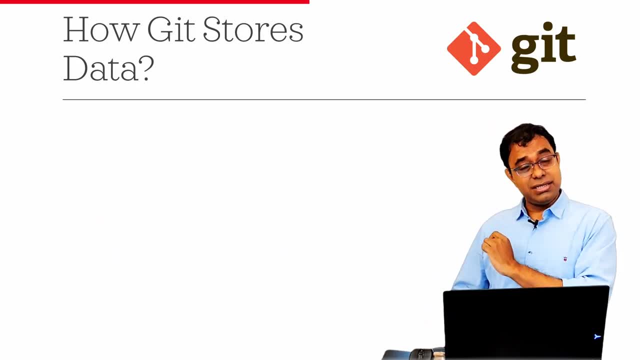 the very important thing about Git- how Git stores data, because this is where Git is different from almost all. Now what Git does is that it Git stores snapshot, not the difference, And sometimes people get confused in this. Let me try to explain with the simplest possible example. Now the other version. 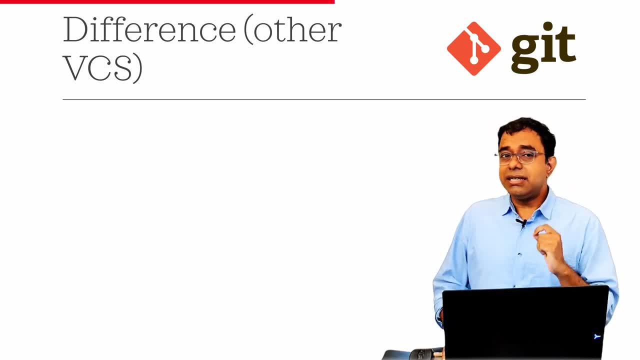 control system store difference: Git store snapshot. So here is how other version control system work. Let's assume that you have a file where it is written this is a test And later on you update the file and write that this is a new test. 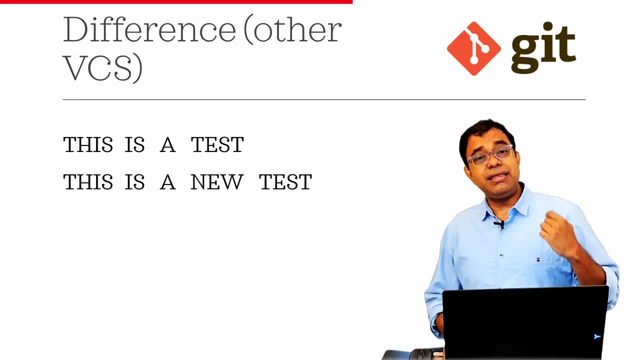 So what other version control system does is that they store delta The difference, which is new. So they will take your original file, match it with the new file and you will get the latest information, latest version of that particular file. Right, 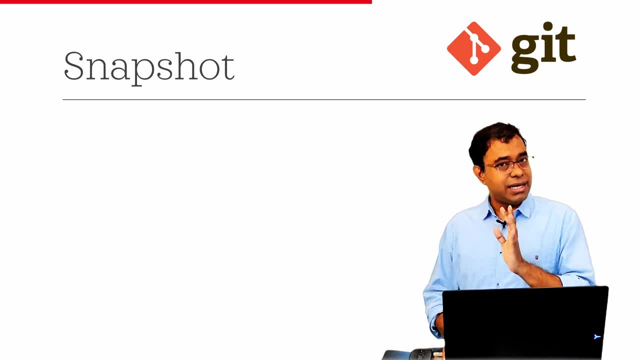 What happened with Git Is that Git takes the snapshot. it doesn't care about difference. snapshot means if your file contains this is a test, this takes a snapshot. you can consider this as a screenshot. right, this is the snapshot, and if you go ahead and change it to, this is a new test, git takes, you know, another snapshot, okay. 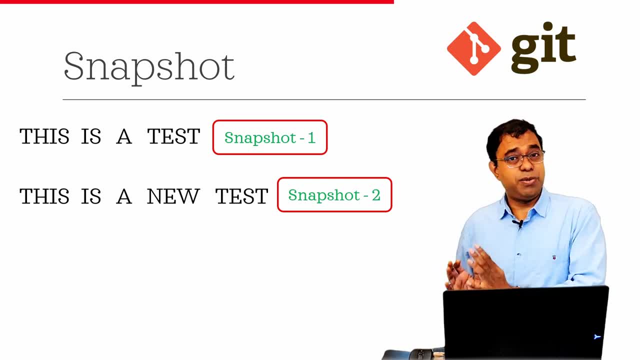 it doesn't maintains the difference. so this is the simplest possible way i can explain the difference between, you know, the delta storage and snapshot storage. git takes the snapshot of whatever is being done at that moment of time when things are committed. of course there are multiple complicated 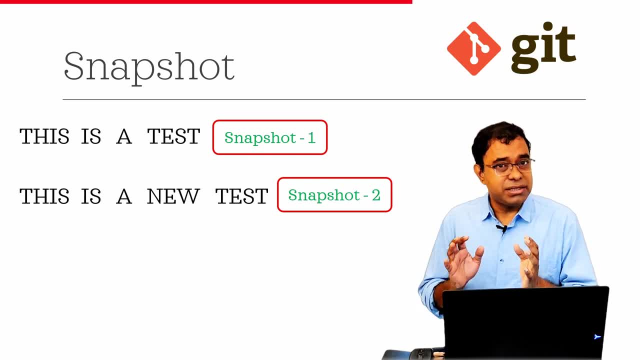 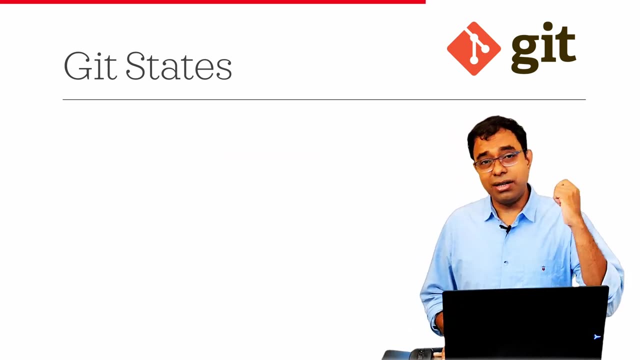 way to make sure that you know this usage and compression is applied. but git works in a way where it takes snapshot. it doesn't stores delta. okay, now the other important thing is git states. this is extremely important if you want to use git. the git states are three prominent states modified. 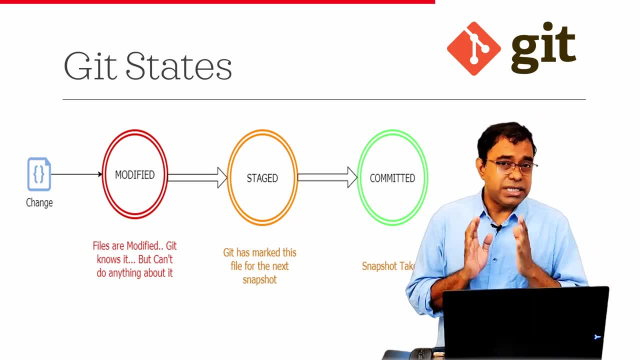 stage and committed. so whenever you change your file in your git repository in your local place where you have changed the file, git knows that the files are being changed. so git says that i know these files are being changed. they are in modified state and i cannot do anything about it. 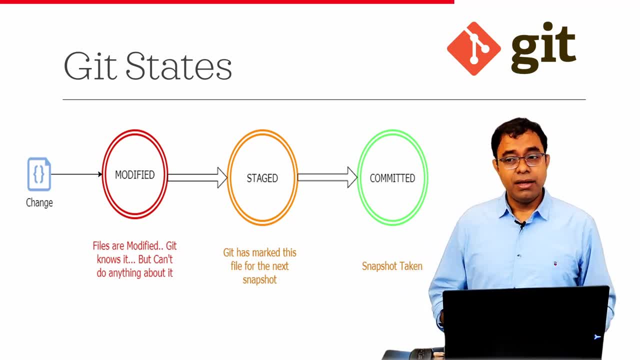 i just know that these files are changed Now. second state is staged, where user says that you know I have changed these files and I want to put it into git and that's the place where you mark your files in the staged. Staged state means that git is telling to the 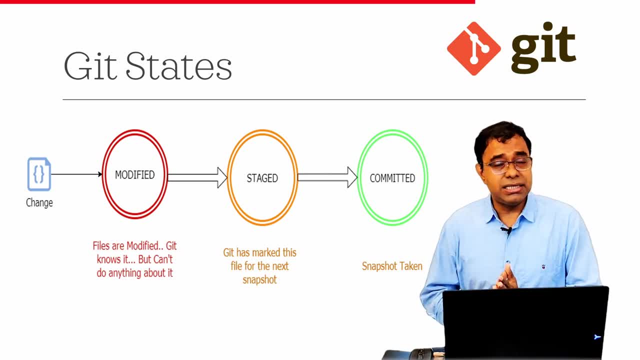 user. you know, I know that these files are being changed and in the next snapshot I will take it: okay, that is the staged state, and later on, committed state. when the committed state happens, git takes the snapshot of the current changes. so these are the three stages. git goes through for any change. for 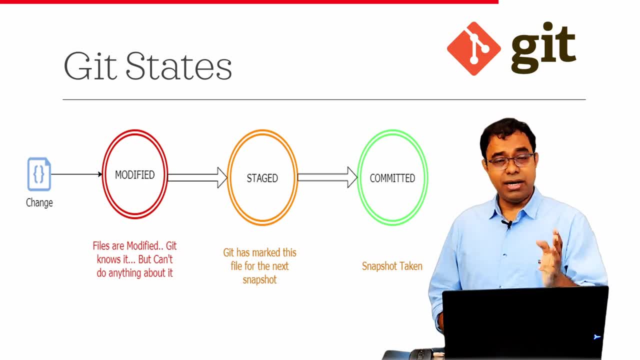 updating any change in any files or directories in the source tree Modified. git knows that it has been modified but can't do anything about it until and unless you put it into staging. then from staging, whenever the next commit happens, git will take the snapshot. Now we have 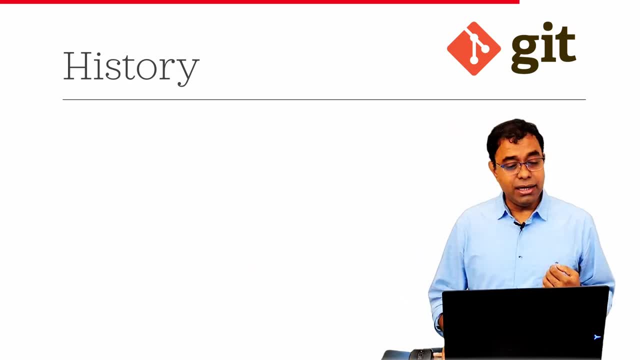 talked so much about git. let's talk about the history of git. Git is developed by Linux community, especially Linus Strobalt, the creator of Linux. it was born in 2005. there is an interesting story out there. you know the Linux community was using some different source control tool called bitkeeper, but 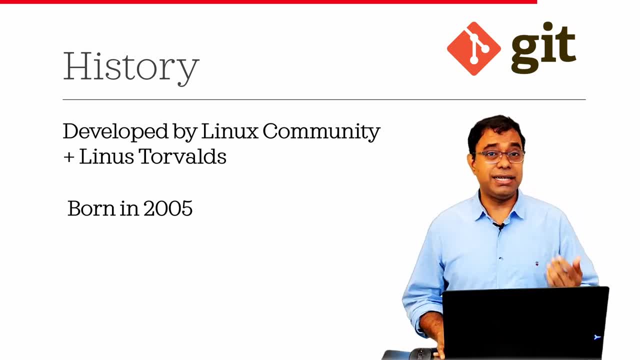 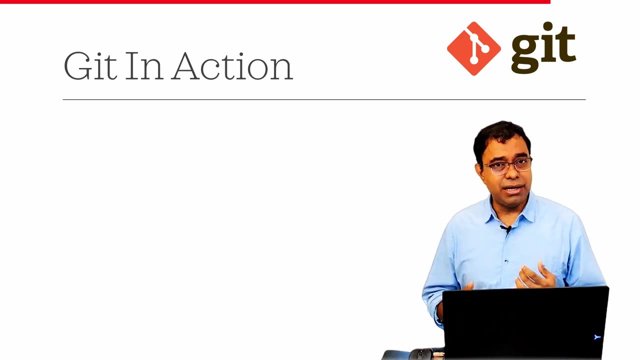 there was some problem that it no longer remained open, so they decided to come up with git. okay, and some of the well-known open source git repository are github and you can also use bitbucket from Atlassian. Now let's go ahead and see how you can install git and what it looks like. okay, so you can. 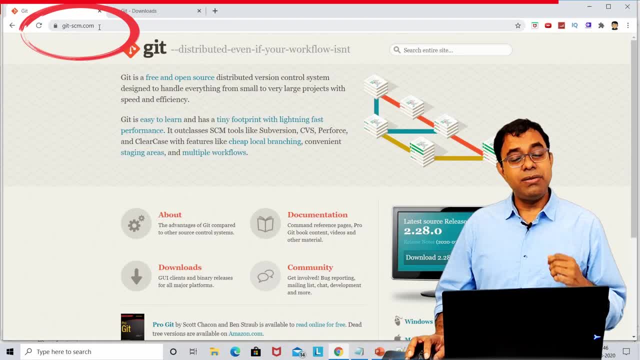 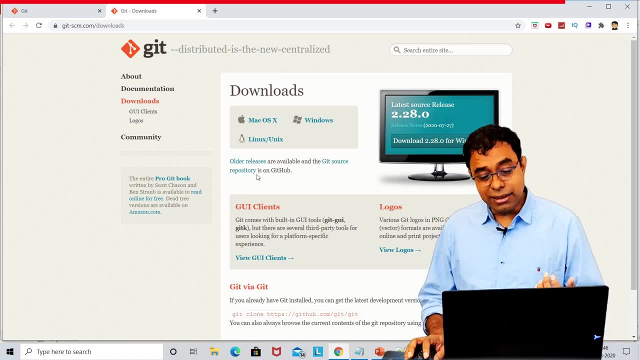 go to git-scmcom. this is the source page of the git. there is a downloads folder. if you come here, you can download git based on your operating system, whether Windows, Linux, Mac. git works everywhere, okay. so this is the latest version which I have downloaded and installed on my system and to verify the installation you.